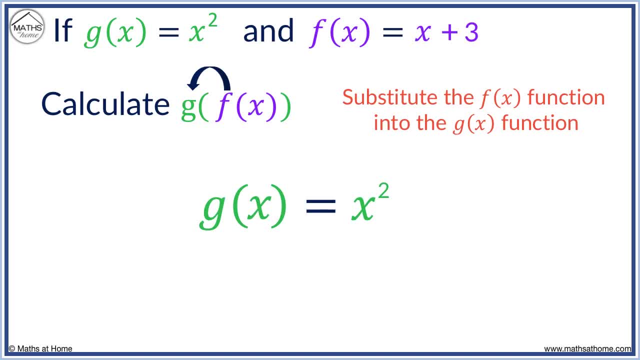 g of x function, which is x squared. To find g of f of x, we substitute x with f of x. The g of x function is squaring x, so we will be squaring also, But instead of x squared we have x plus 3 squared. We replaced the x with x plus 3.. Notice that we need brackets. 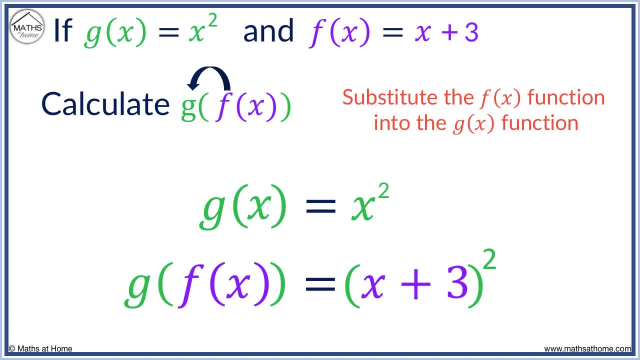 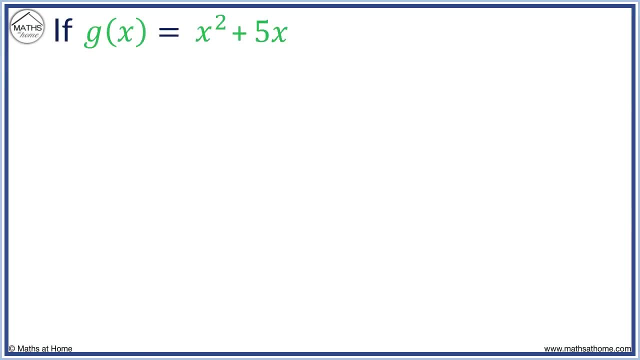 around x plus 3, because we are squaring the whole thing Here. if g of x equals x squared plus 5x and f of x equals the square root of x, calculate g of f of x Using the backwards arrow f. 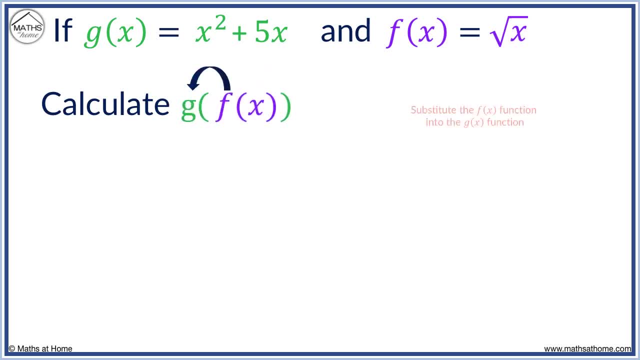 of x is substituted into g of x, We start with the outer function. g of x equals x squared plus 5x. To form g of f of x, we replace the x's with f of x. This means that every x in the g of x function is replaced with the square root of x. The 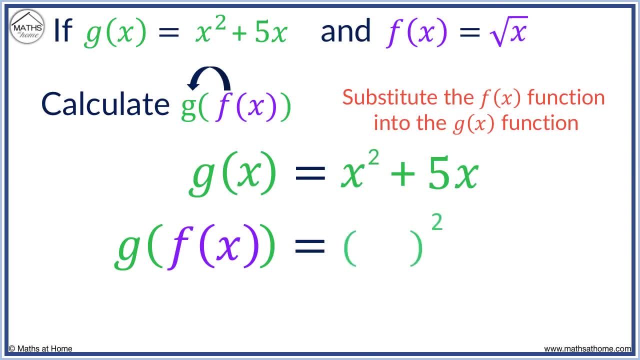 first x is squared, so we put a bracket squared, But instead of x we put the square root of x. We then have plus 5.. And instead of x we have the square root of x. Both x's have been replaced with the square root of x. 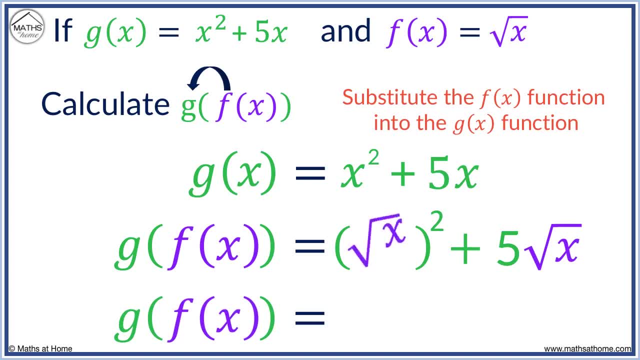 We now can simplify: The square root of x and the square functions are inverse functions which can cancel out The square root of x. squared is just x. We then have plus 5 square root of x, g of f, of x equals x plus 5 square root of x.